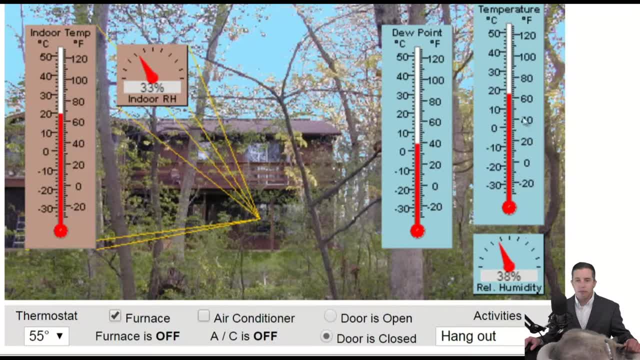 mixing ratio in it, but it's the same concept. So right now the temperature is a little bit above 60 degrees, The dew point looks like it's a little below 40 and our relative humidity is 38%. Okay, so if I raise the temperature, so I just drag this up- notice what's happening to the relative 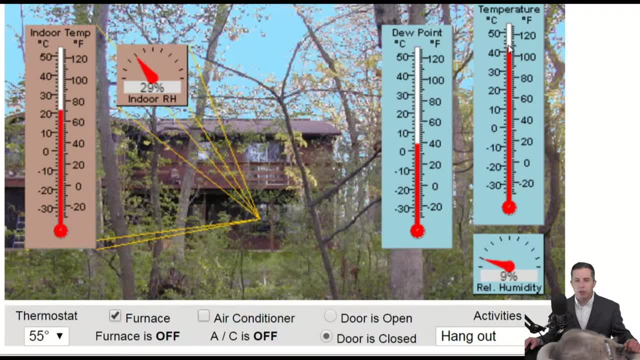 humidity. as a temperature goes up, the relative humidity goes down. So to relate this to what we've done before with mixing ratios, we said the top of the fraction was the current mixing ratio. That's not changing because dew points not changing. Remember dew point mixing ratio. 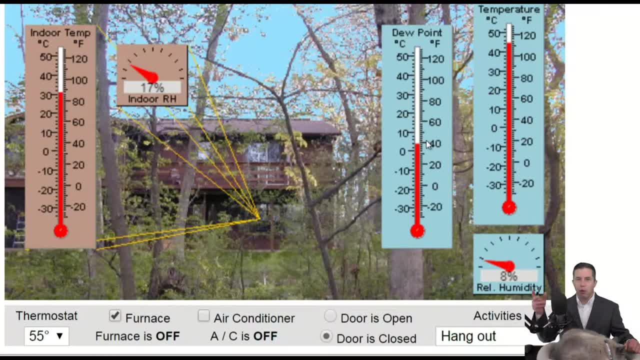 have to change together. If I add more water to the air, they both go up. If I subtract water from the air, they both go down. The fact that dew point is not changing tells me that the amount of water in the air is still a constant. But I increased the temperature. 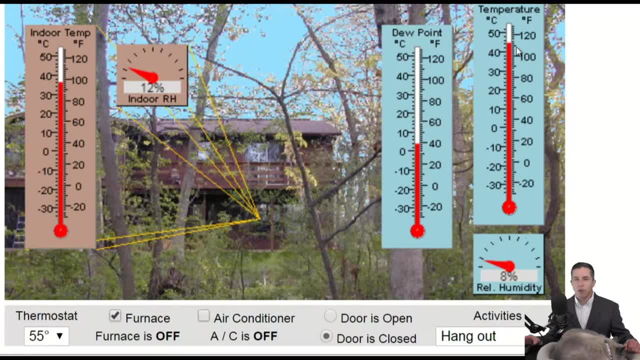 just then. And so again, to relate that to what we've seen before, I'm dividing by the maximum possible mixing ratio, and the maximum possible mixing ratio goes up as temperature goes up, And by a bigger number gets me a smaller answer. So as I raise the temperature, you saw the. 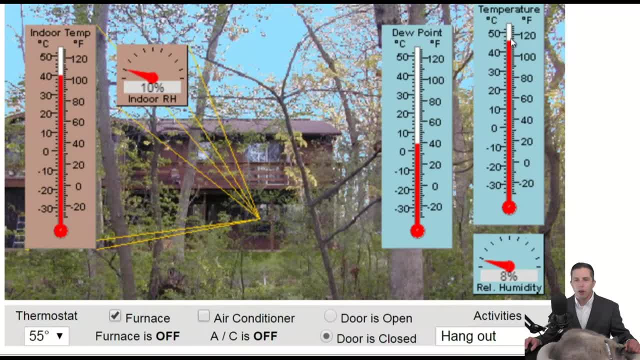 relative humidity decreased. So I will continue to raise up the temperature. We'll make it as hot as we can make it. Relative humidity goes down to 5%, Okay, so watch what happens when I cool it down. So I'm going to cool down the temperature. So I cool it down and 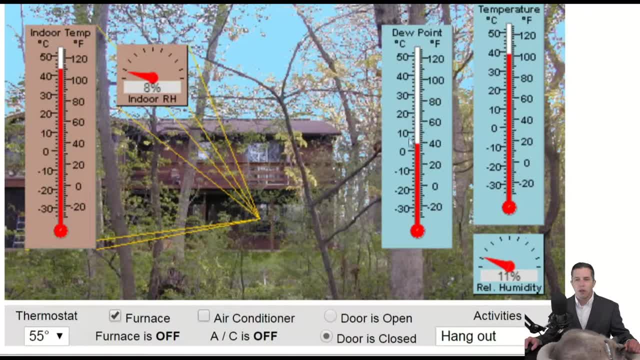 I cool it down and notice the relative humidity is increasing. The dew point is not changing because I'm not taking water from the air. Okay, so I'm going to drop it down, Drop it further, Cool it, cool it and notice that the relative humidity continues to go. 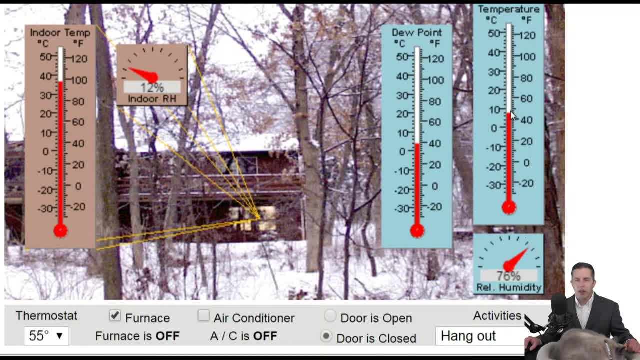 higher and higher. And so now, as I, as I'm getting closer and closer to the dew point, the dew point is a little below 40. I'm getting, I'm getting close. Notice how high my relative humidity is, So I'm going to drop it even further, Drop, drop. Okay. so now relative. 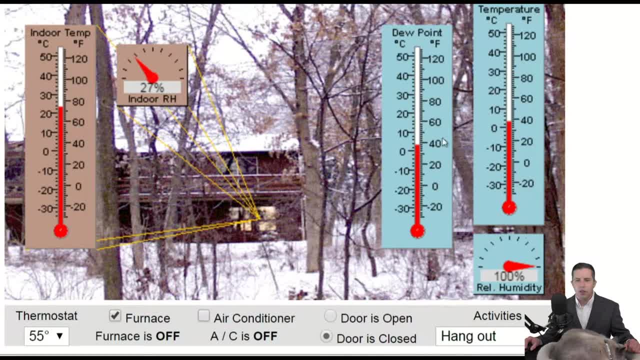 humidity is 100%, Temperature and dew point are the same. Okay, so I'm going to continue to cool it further. So we would be making dew at this point, even though the picture shows snow. That's not quite correct, because we're above freezing, but we would be making. 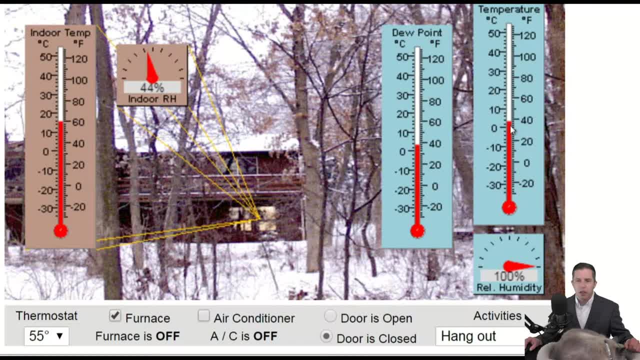 dew. Okay, so I'm going to, I'm going to- lower the temperature. So as I lower the temperature, notice what happens to the dew point. The dew point has to go down with it, but the relative humidity stays at exactly 100%. Right, so I can now we're below freezing for sure. 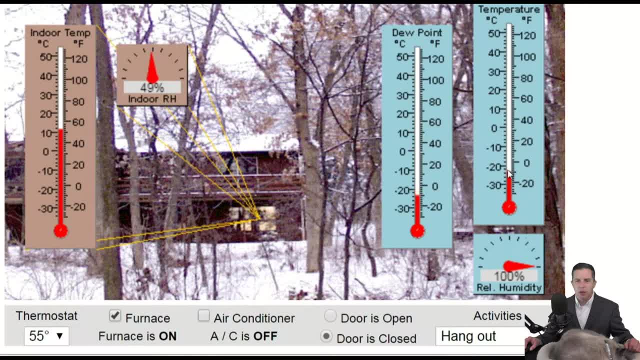 We're making frost, but I'll keep going down and keep going down, Keep going down, Keep going down. And as long as I keep making it colder and colder, the dew point has to go lower and lower, because I'm taking water out of the air and putting it onto the ground. 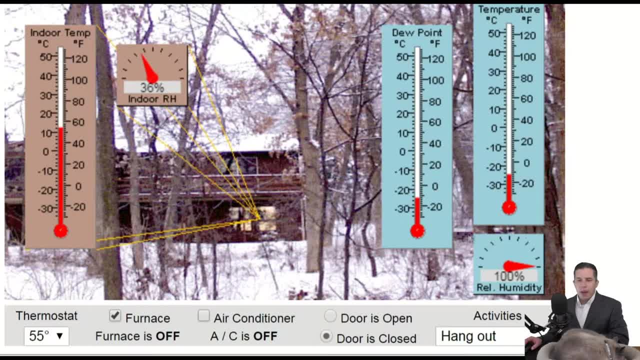 At first it was liquid and then it's frozen, But that entire time the relative humidity was staying at 100%. So now, let's say I warm it up. So now the dew point is really low. The dew point looks like it's about negative 10.. And as I warm the temperature up, you 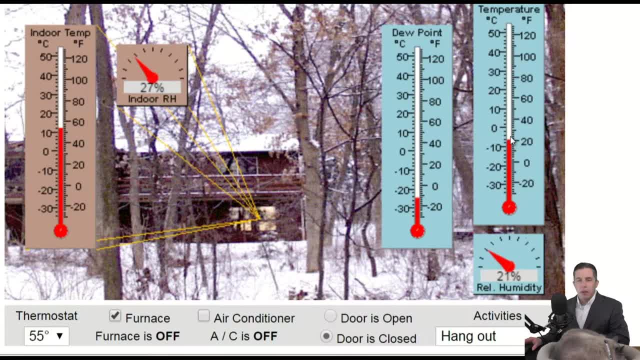 can see that relative humidity rapidly drop. Now this is not completely realistic, because normally what happens? if you, if we made do in the more overnight and the dew sitting on the grass, then when the sun comes up the next day, that do evaporates back into the. 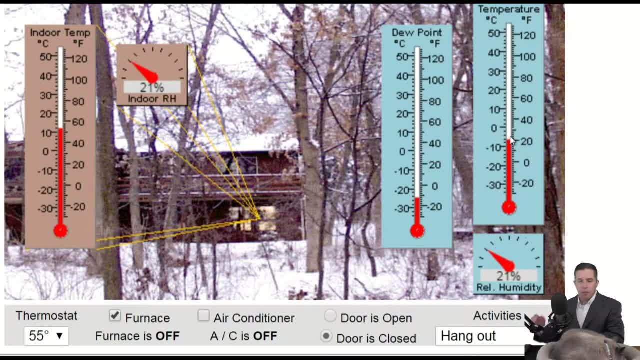 air- at least most of it does- And the dew point would go back up. What this is doing is, once we lowered the dew point, it's keeping it lowered right. So that's not quite what happens in nature usually. So here's another thing I could do. So let me crank up the temperature to 60.. Relative. 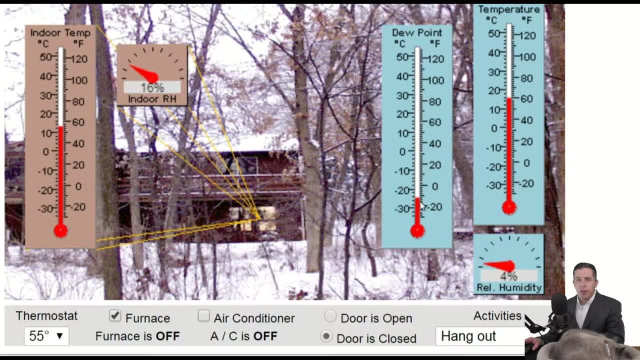 humidity is 4%. If I add water to the air I increase dew point. right, So I can crank up the dew point. As I crank up the dew point, relative humidity is also increasing. Now, in this case it's increasing because we think again back to the definition of relative. 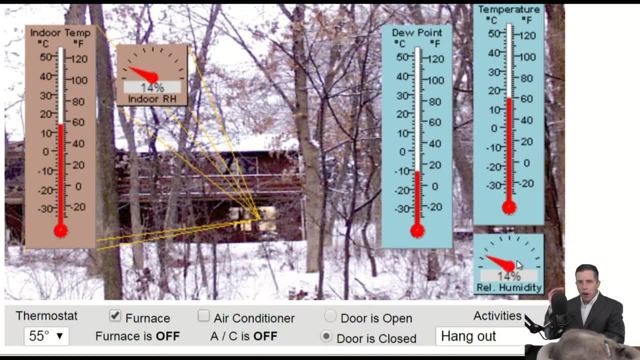 humidity that we use with. with mixing ratios, The top part of that fraction was the relative humidity. That's the current mixing ratio. How do you increase the current mixing ratio? You add more water to the air. You add more grams of water to the air, Increasing dew. 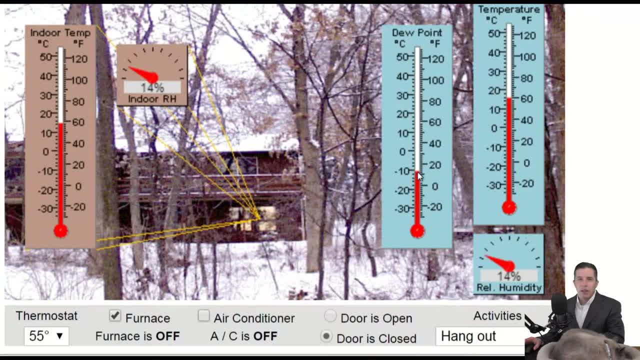 point is the same thing. If I add water to the air, dew point goes up. So we don't see a process here. You have to imagine there's someone off the screen that's adding water to the air somehow as I crank this up. So there's some mechanism that we can't see that. 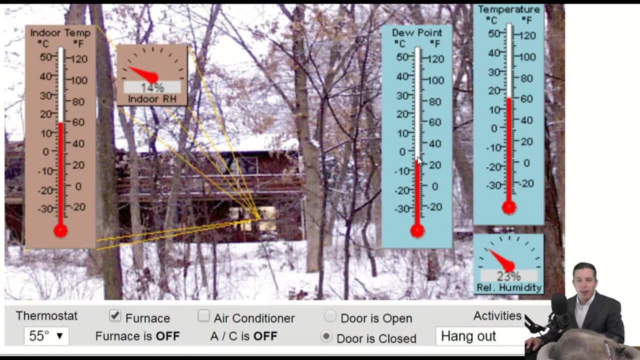 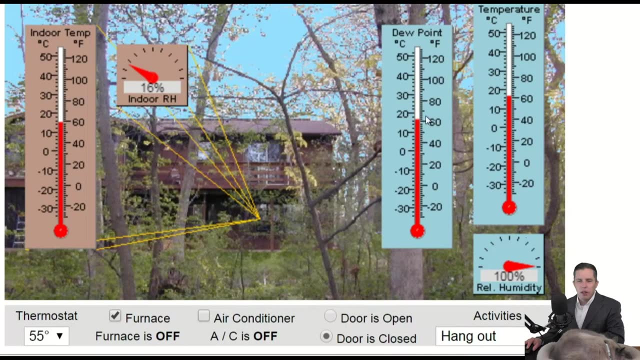 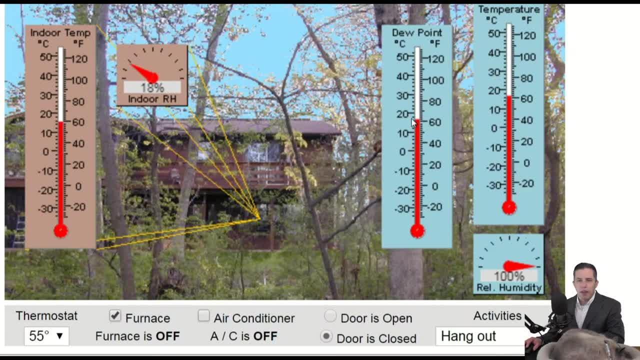 humidity, temperature and dew point are the same. if i, it is physically impossible for me to have dew point above temperature. so the way this software handles this is: if i try to crank dew point higher, it also just raises the temperature. so that you don't have math that makes no sense. 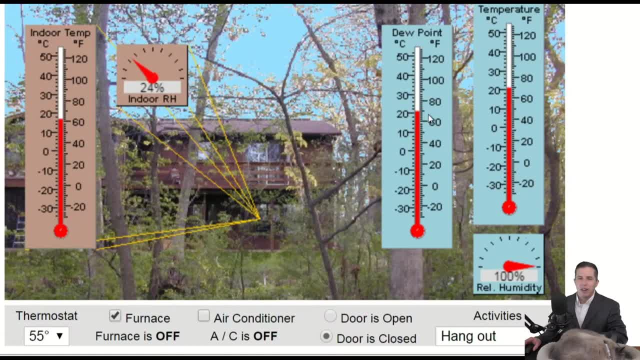 but in reality if i was actually adding water to the air, the temperature does not magically go up. okay, that's kind of a limitation of this, of this software simulation. so here: dew temperature: 80 degrees. dew point: 80 degrees. relative humidity: 100. this would be a pretty. 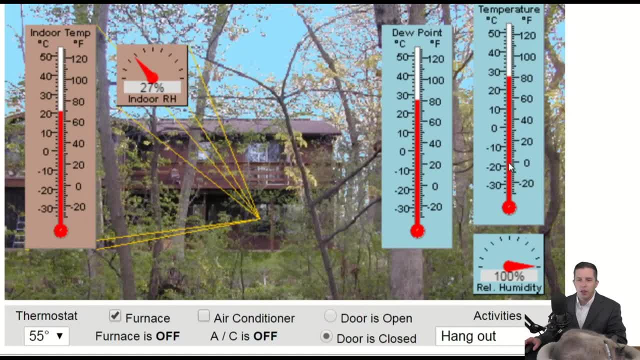 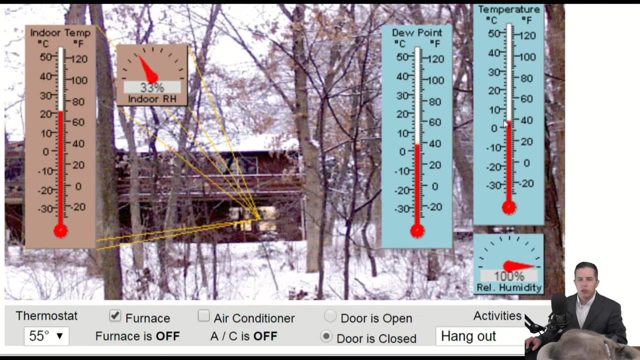 miserable place to live right now. if you had this, because you, as we talked about, with the evaporation lecture, your sweat would not evaporate. so from here, if i cool it down, i'm generating a condensation, make and do making, do making, do. a relative humidity again stays at 100, then i can raise the temperature back up and again the dew point stays. 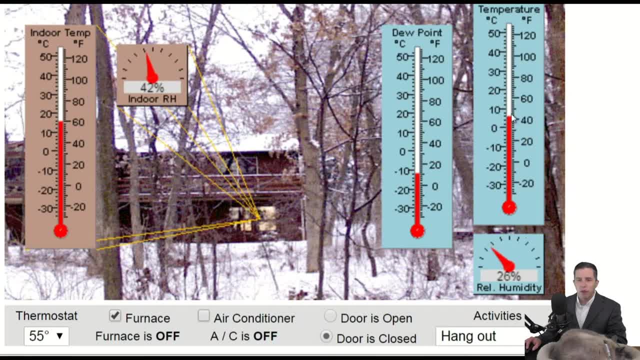 there because we have no mechanism to add or subtract water from the air. so this is a little tool that you can play with. maybe it'll help. on the left hand side. i'm going to go ahead and look at the outside. there is another thing where what they're doing is they've got an indoor. 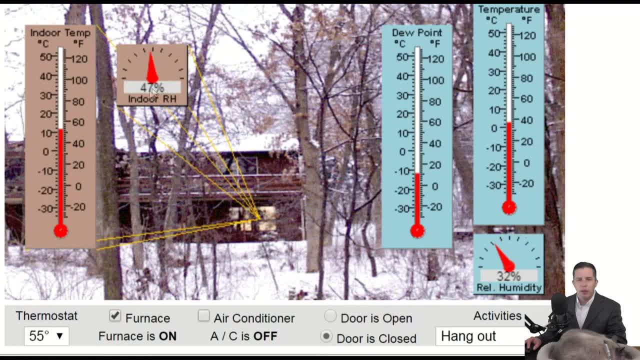 thermometer. so so both of these things are outdoor. there's an indoor thermometer and then indoor relative humidity and you can do things like you can change the temperature, you can turn the air conditioner on and off and you can see what the effect is on the indoor relative humidity. so you 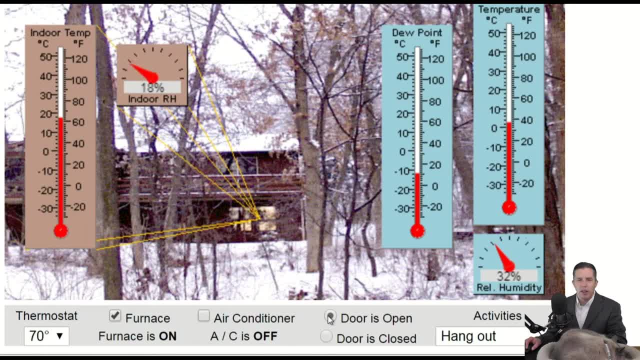 can play with that. if you want, you can open the door and let in some outside air and see how that changes. the the point being that, um, often we have the same air outside as we have inside. right, it's usually the same air, and if i have a relative humidity gauge inside, it'll have one reading on it and i have a relative.